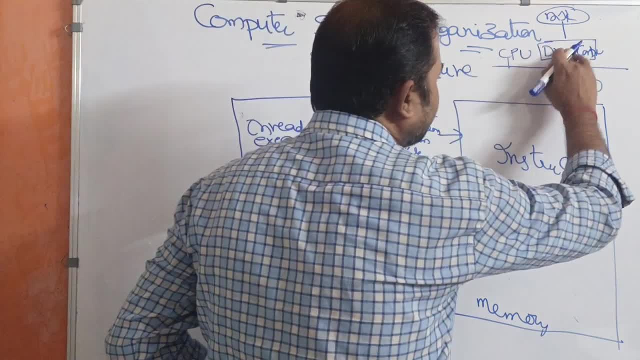 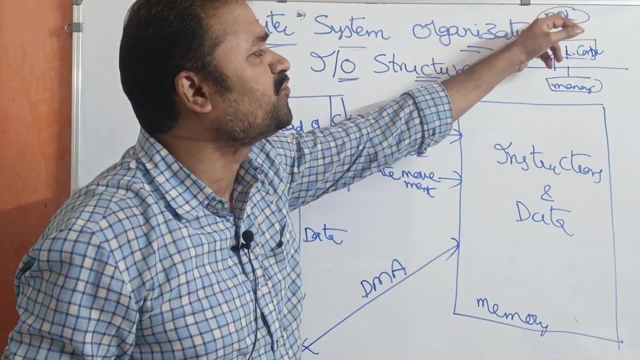 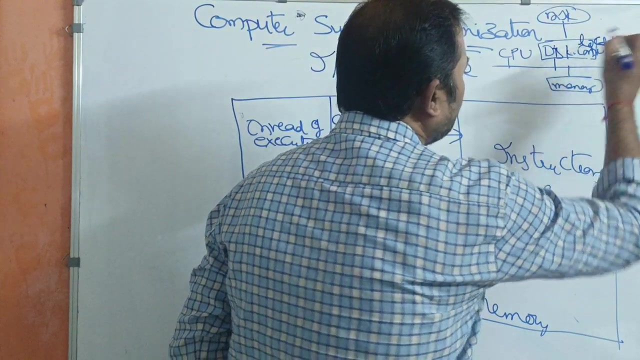 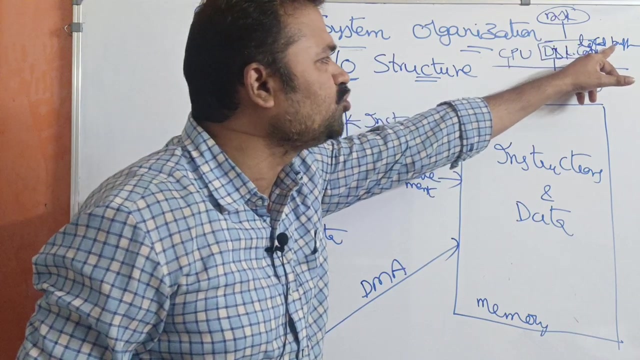 So here, if you take this as the disk controller, Why? because here we have hard disk. Disk controller is in charge of hard disk Disk controller has local buffer which can store the data Here. the data which is in the hard disk will be transferred to the local buffer of the disk controller. 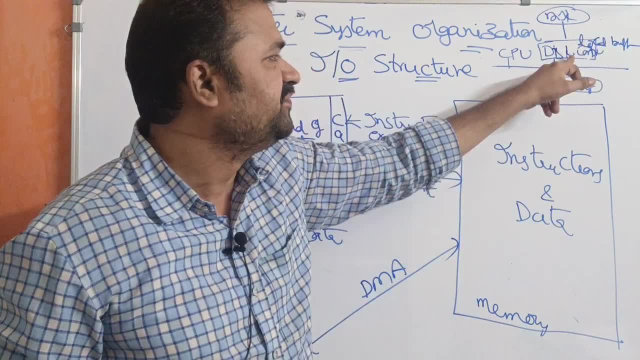 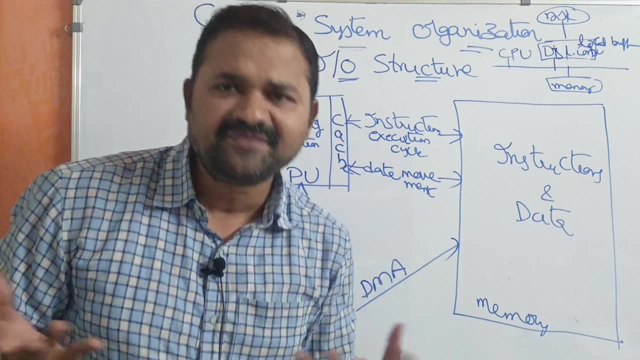 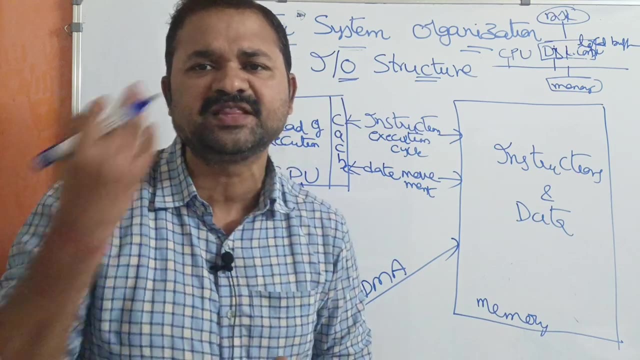 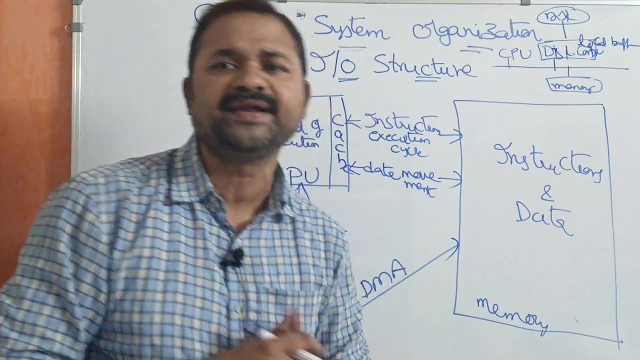 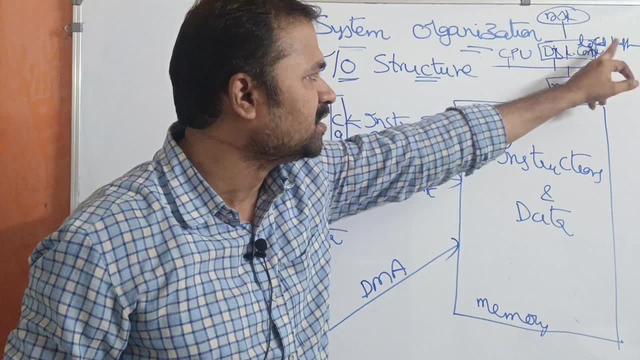 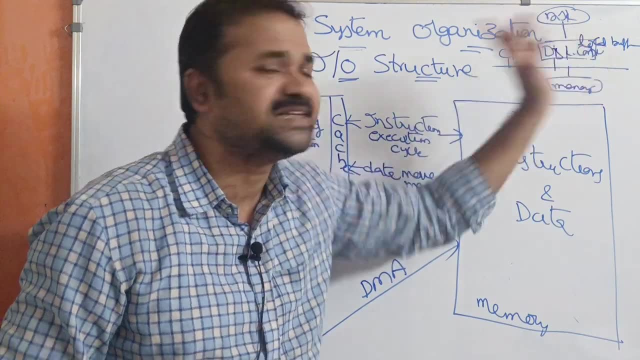 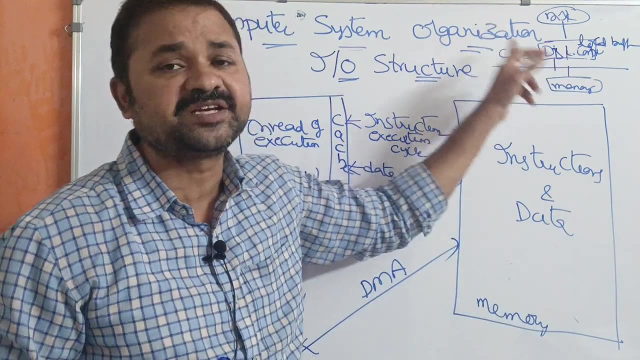 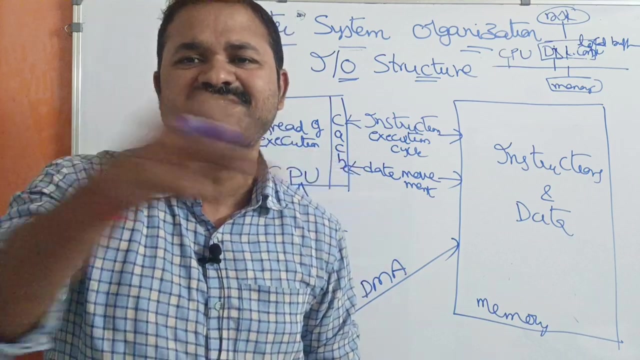 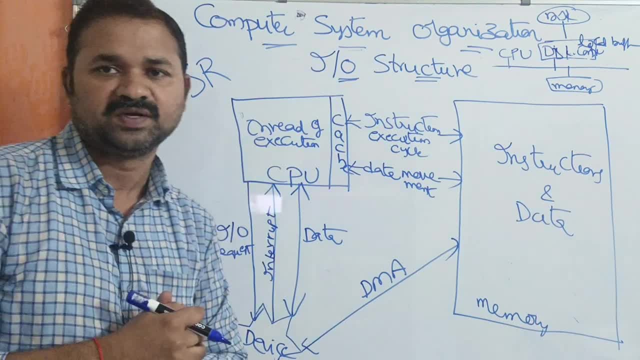 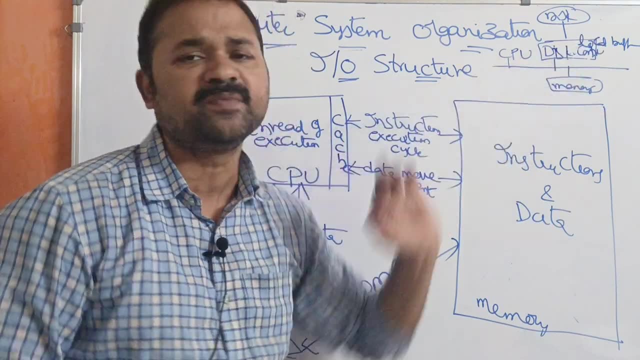 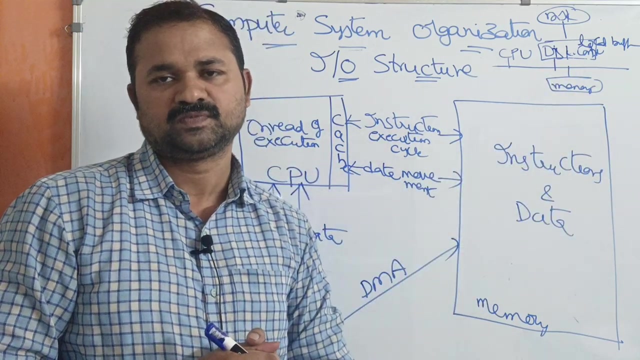 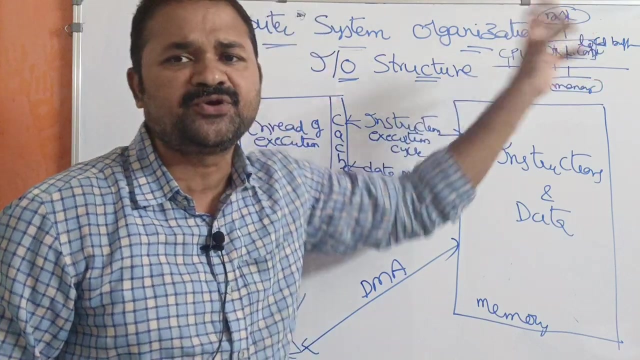 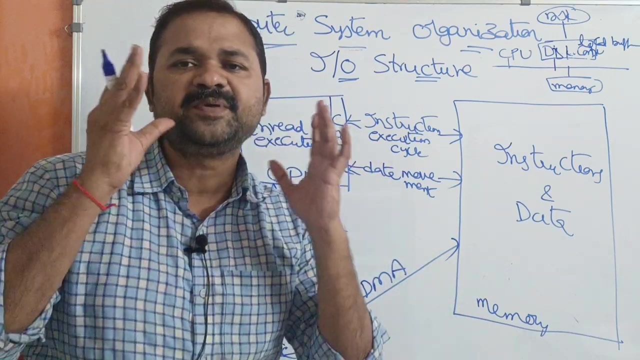 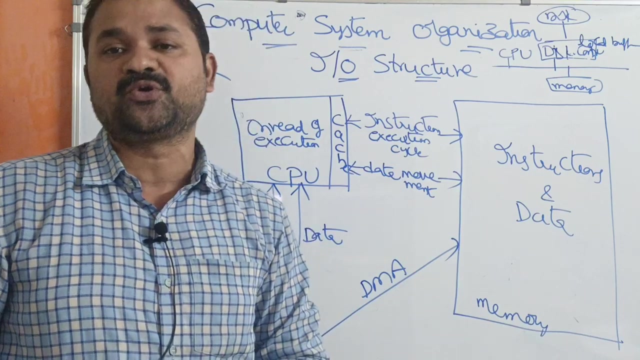 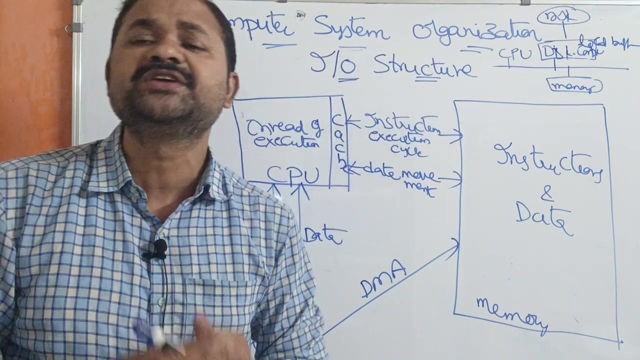 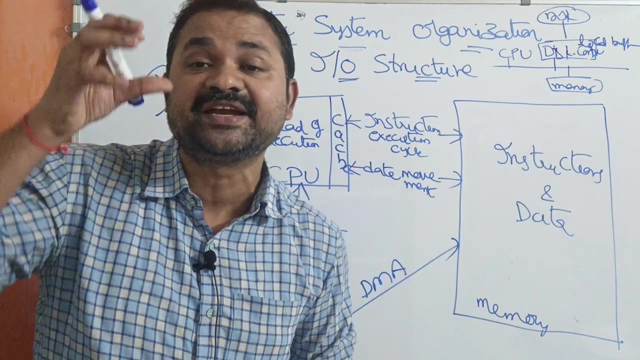 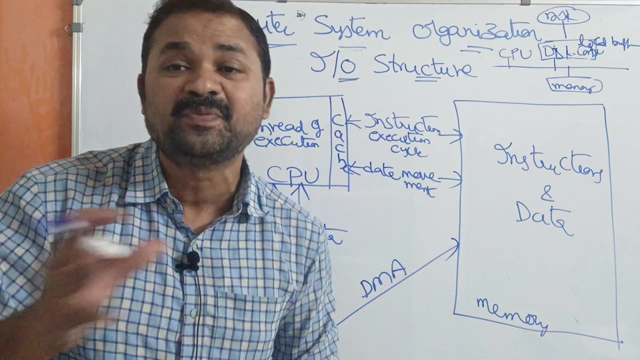 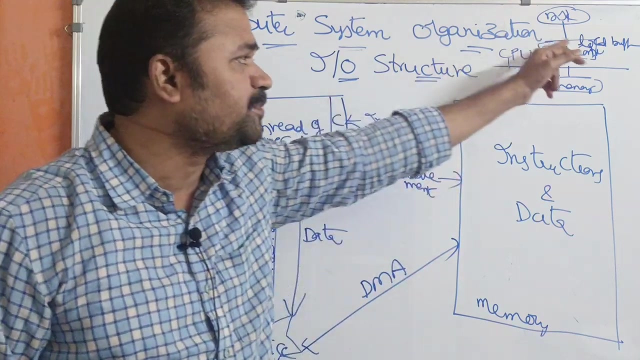 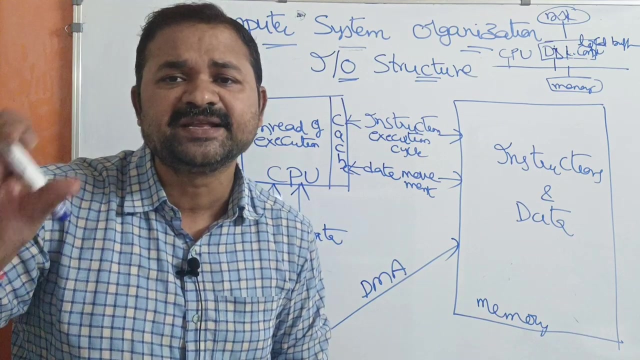 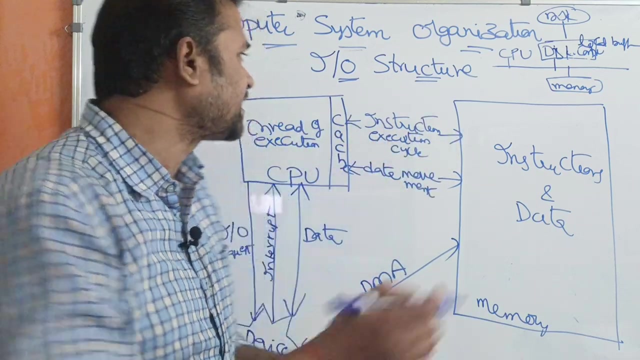 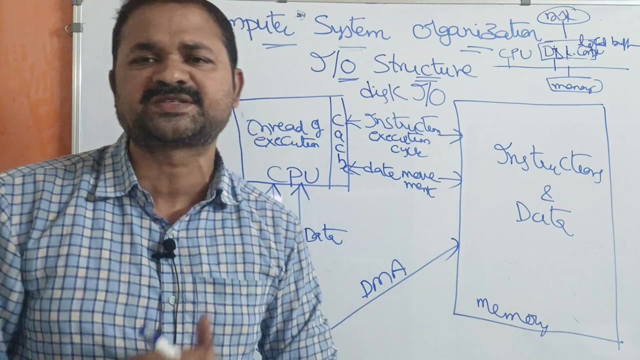 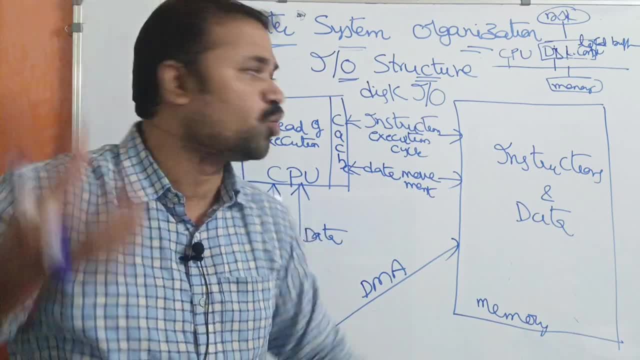 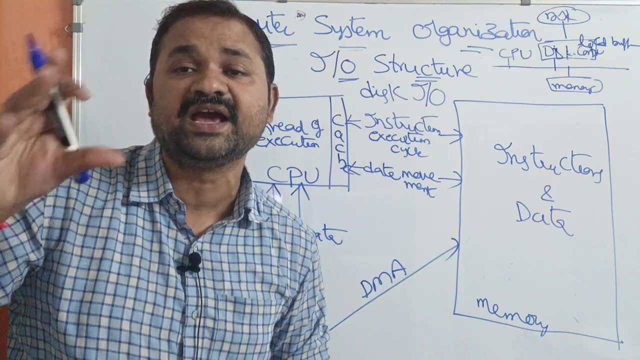 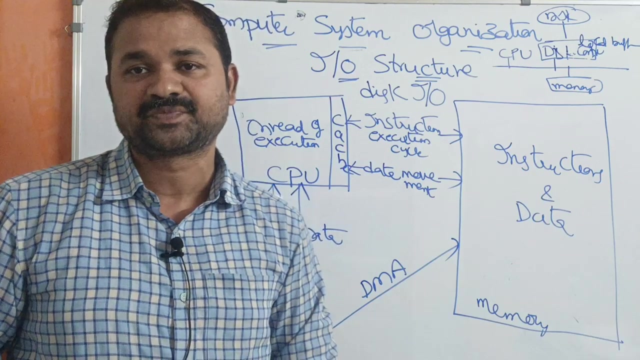 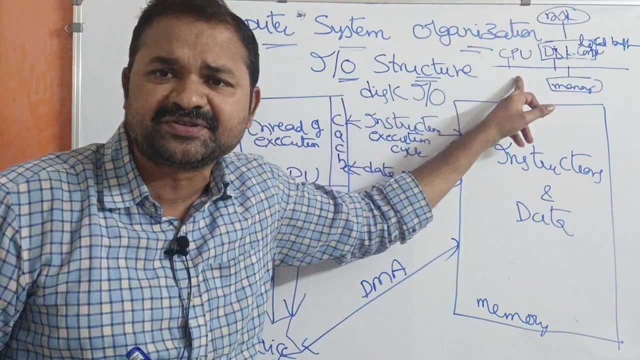 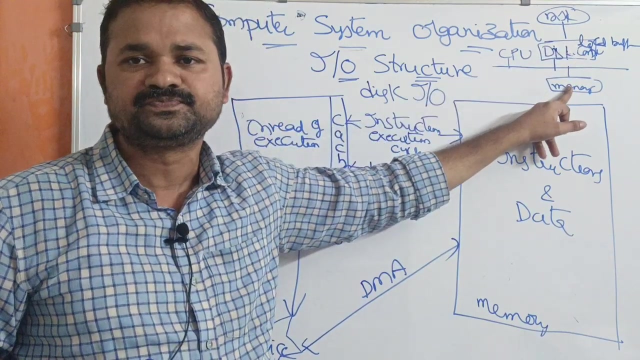 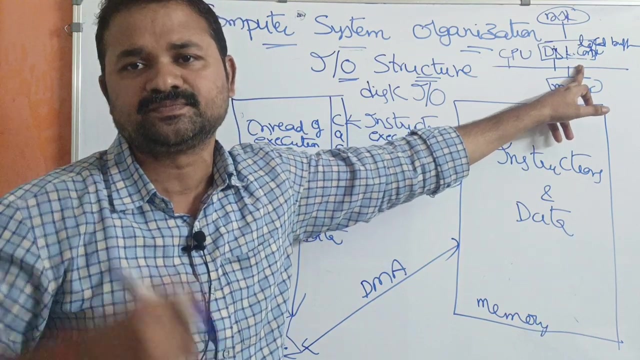 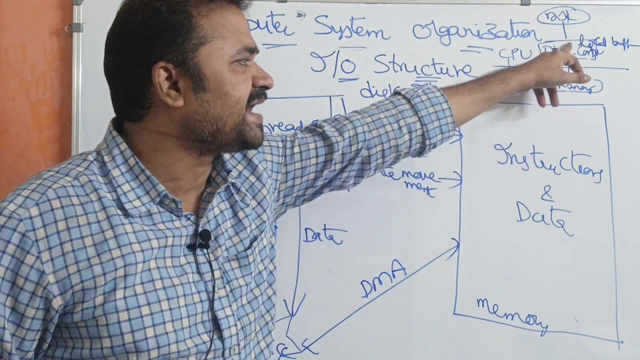 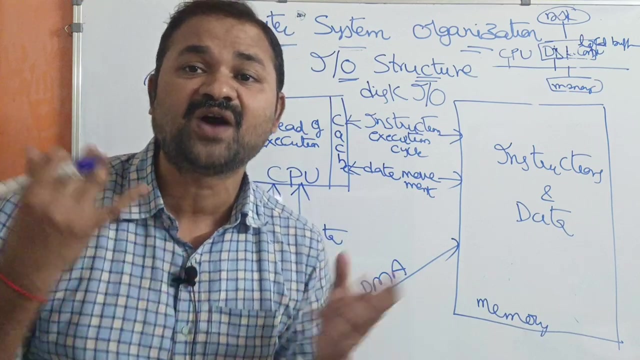 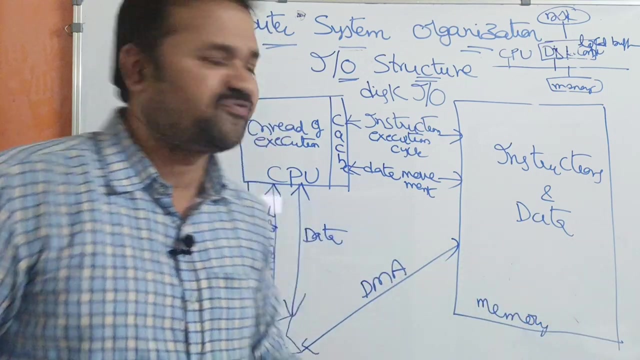 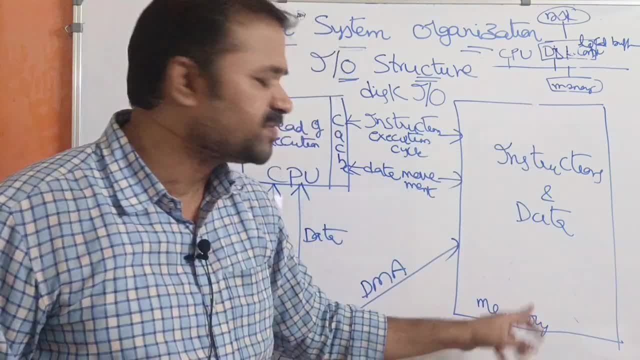 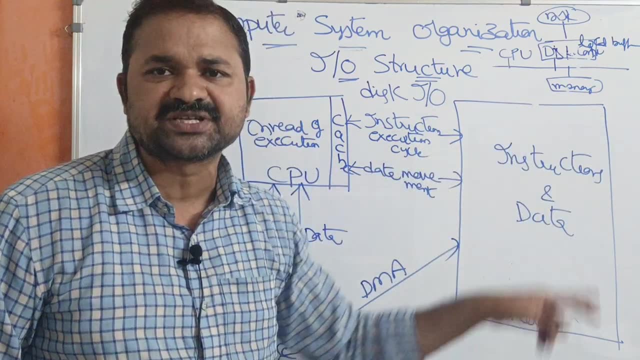 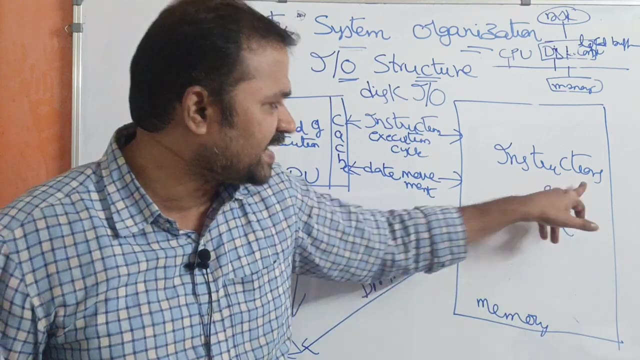 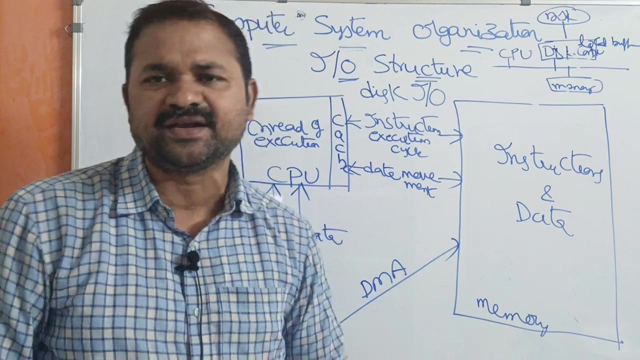 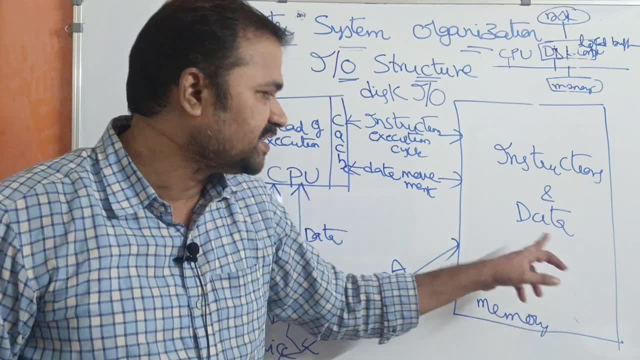 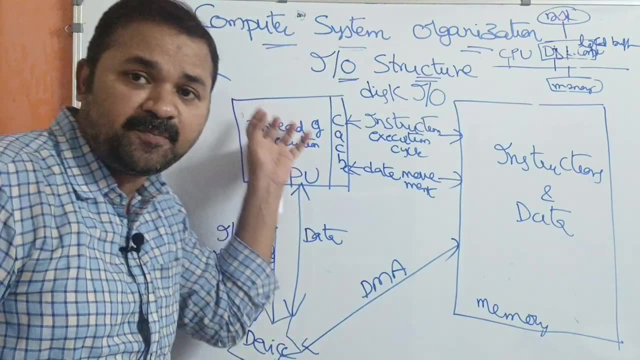 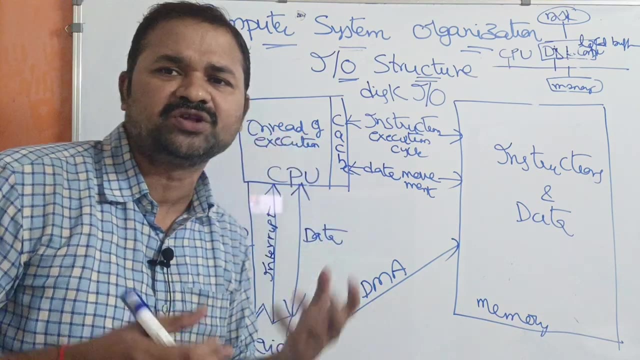 values 10, 20, 30, 40, 50. so that is nothing but data. so this is main memory and this is nothing but cpu. this component is nothing but cpu. here we have catch memory, catch memory and thread of execution. we know that cpu executes the programs, instruction by instruction. here cpu fetches. 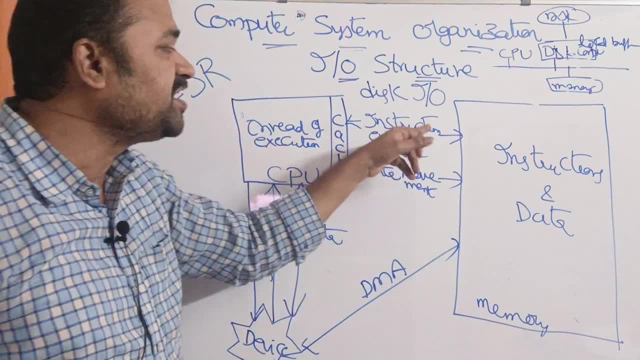 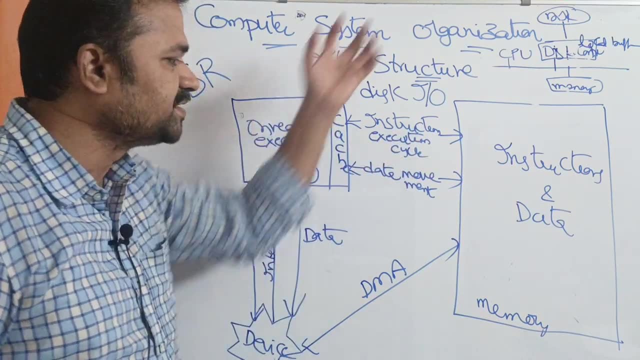 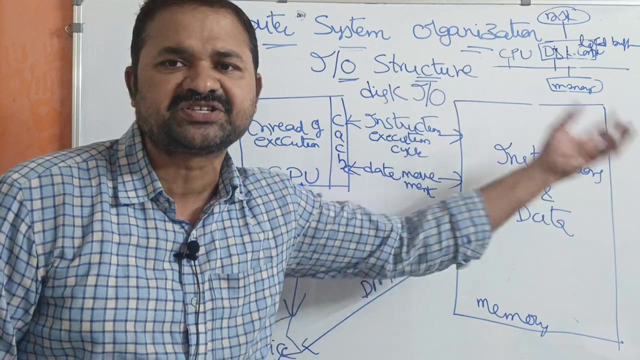 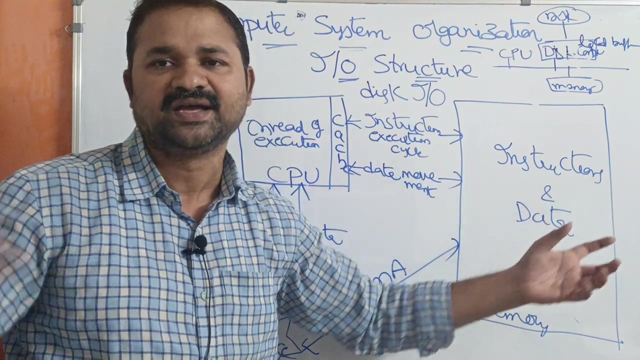 an instruction from the main memory and it will execute the instruction. so this is nothing but instruction execution cycle. so cpu fetches an instruction from the memory and it will execute that instruction. likewise, instruction by instruction will be executed and data will also be moved. so cpu wants the data, a value data, in order to execute that one, so that data. 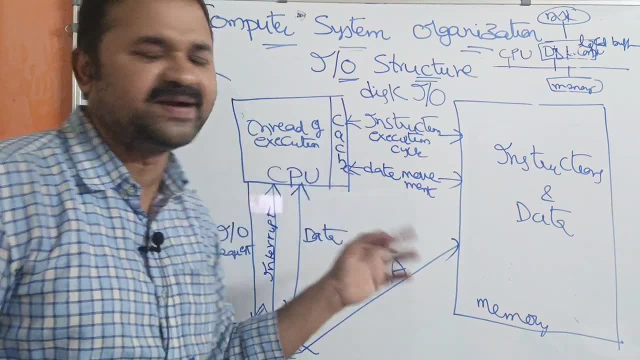 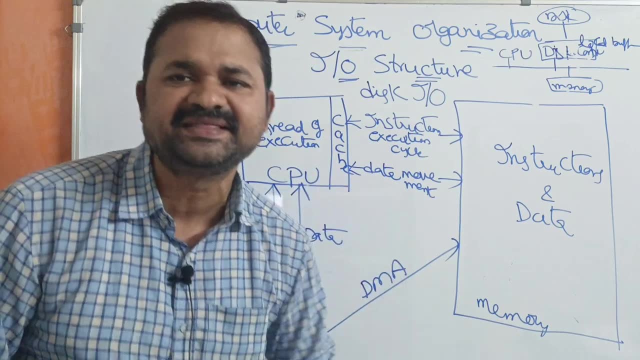 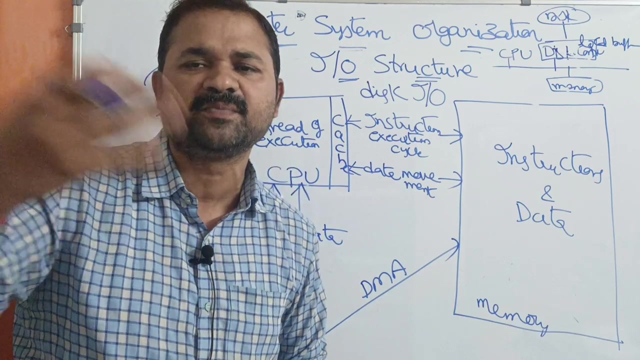 can also be moved. so. So this is nothing but cpu, so this is nothing but thread of execution. so here cpu executes any task thread by thread. we know what is a thread. thread means a small unit of execution. so cpu executes that program thread by thread. next, here we have device. so this device may 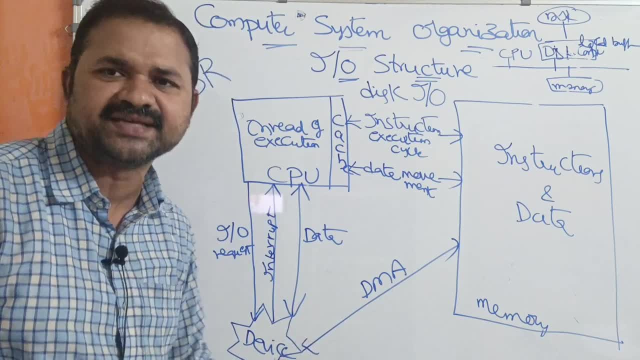 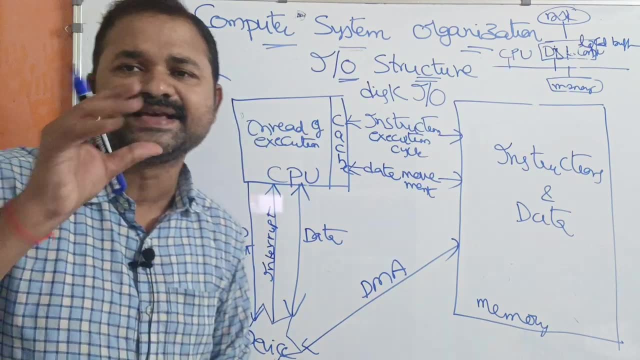 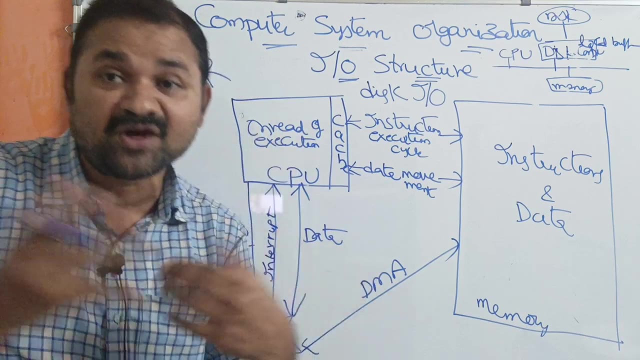 be any device. it may be input device or output device or hard disk. it may be any device. so here the cpu is executing the program. while Executing the program, it finds an IO request. like we use a scanner function in C language, We use a printer function in C language. 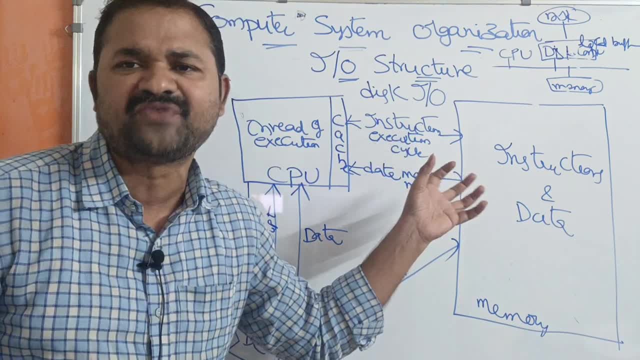 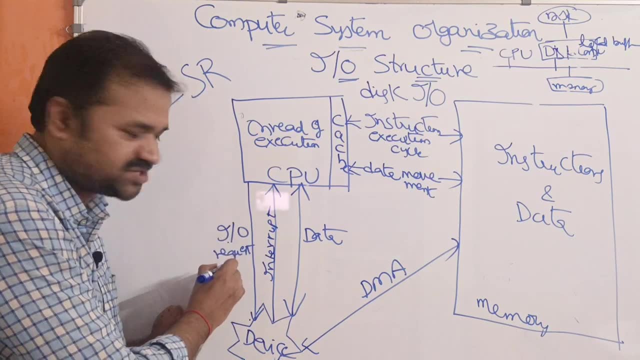 Those are nothing but some IO statements. So whenever CPU finds an IO statement, then it sends an IO request. It sends: this is nothing but IO request. CPU sends IO request signal to the device. 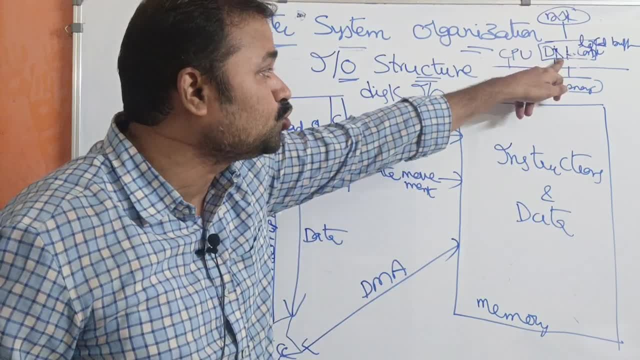 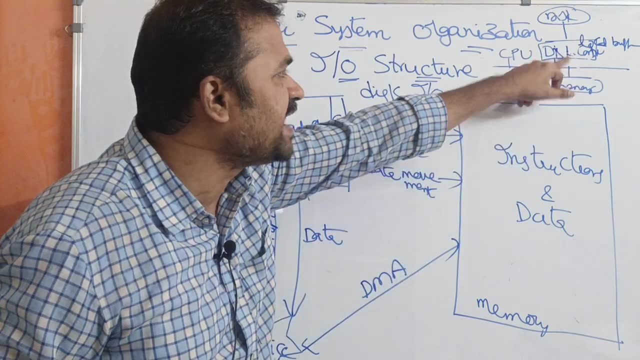 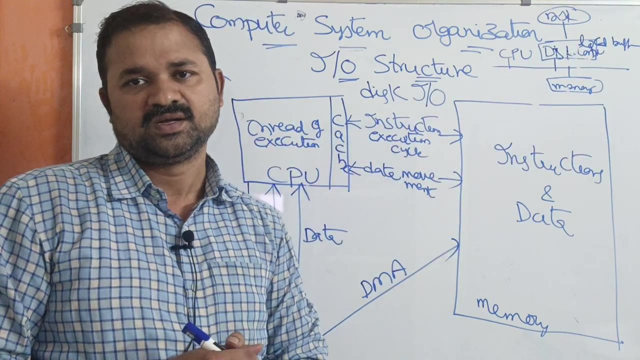 Then the device has to read the data. Let it be the disk request. So now the device has to read the data from disk and the data will be stored in local buffer of the disk controller. So let us assume that now the data is available at the local buffer of the corresponding device. 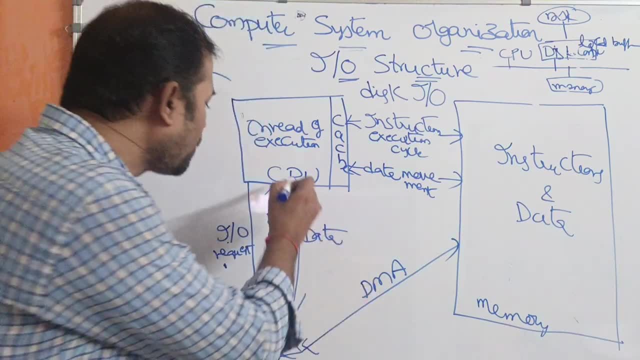 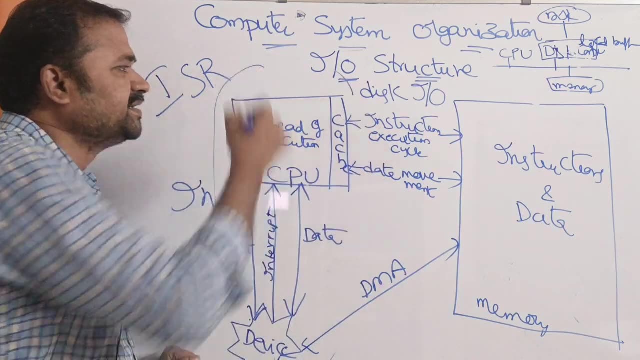 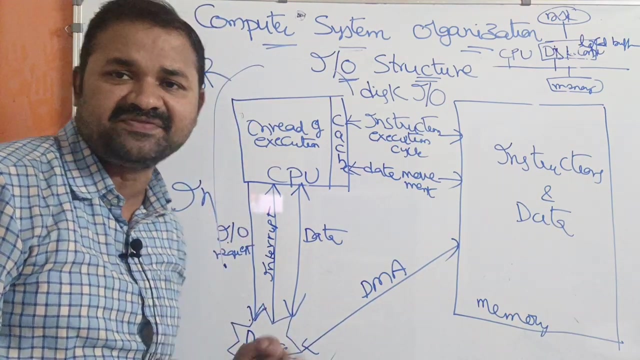 So once the data is available, this approach is nothing but interrupt initiated. This approach is nothing but interrupt initiated IO. This whole diagram, this part, is nothing but interrupt initiated IO. Already we have seen interrupt initiated IO. So once the data is available at the device, then the device will sense an interrupt. 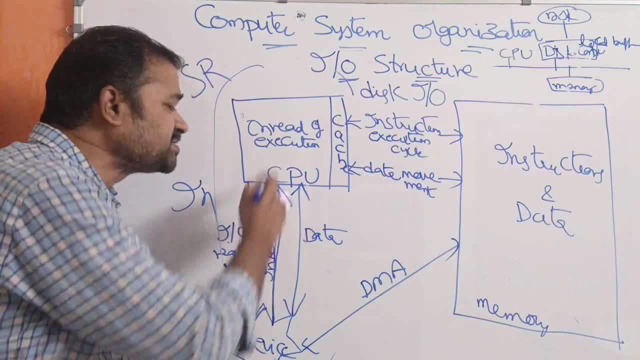 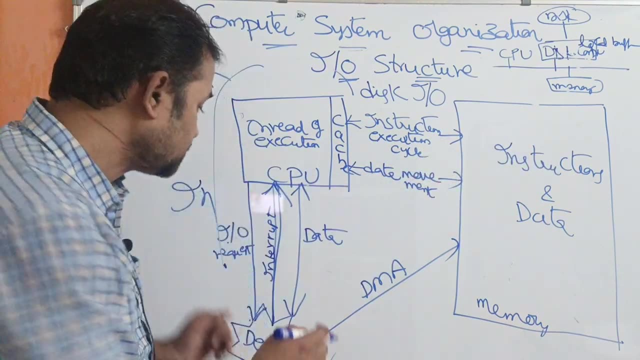 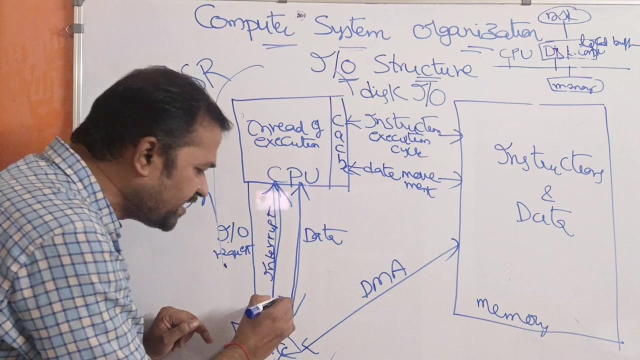 This is nothing but interrupt signal. The device will sense interrupt signal to the CPU. Now CPU has to transfer the data from device into the main memory, So CPU will transfer. yeah, this is nothing but data. So data will be for data. we have IO towards the device as well as IO towards the CPU. 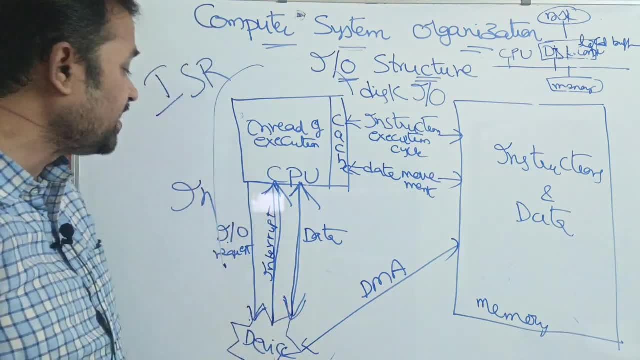 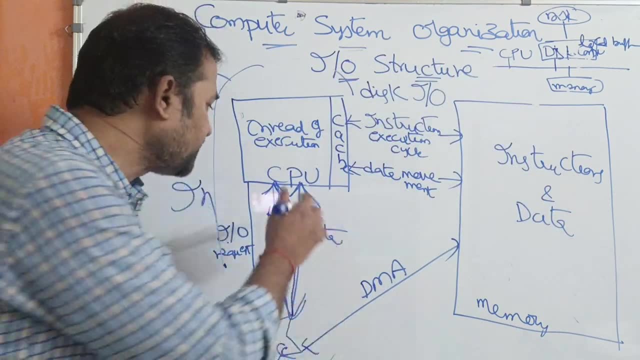 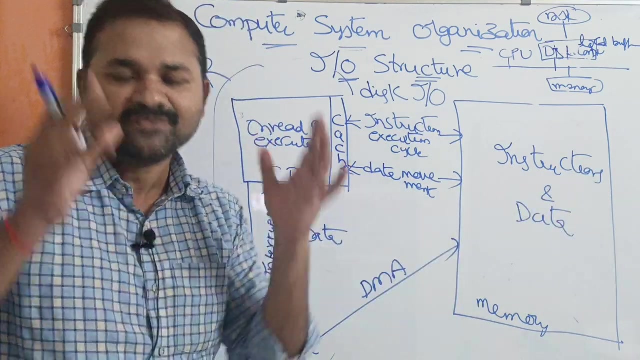 Why? Because here, whenever the data is available, then what the CPU will do? CPU will transfer the data from device to the main memory. So that's why IO will be towards the CPU. But once that program execution is over, then we know that main memory contains only the data that is needed by CPU. 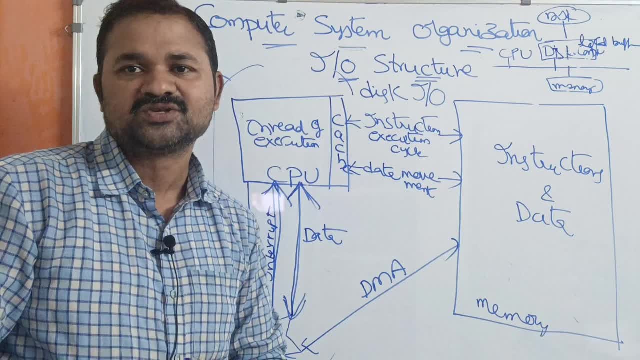 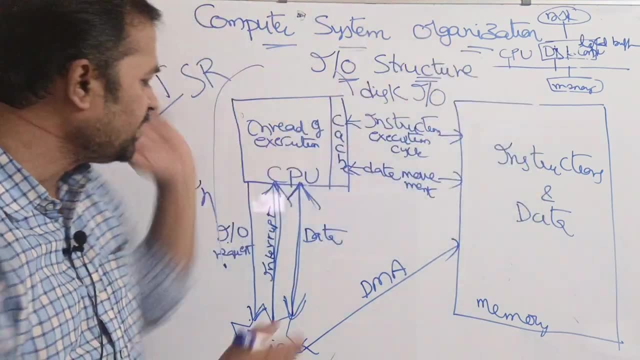 So CPU Executed that program- the data. So once again the data has to be transferred to the hard disk. So once again, CPU transfers the data from that main memory into the hard disk. So that's why IO will be towards CPU as well as device. 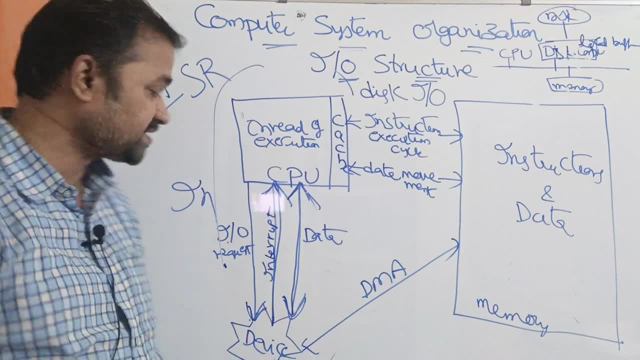 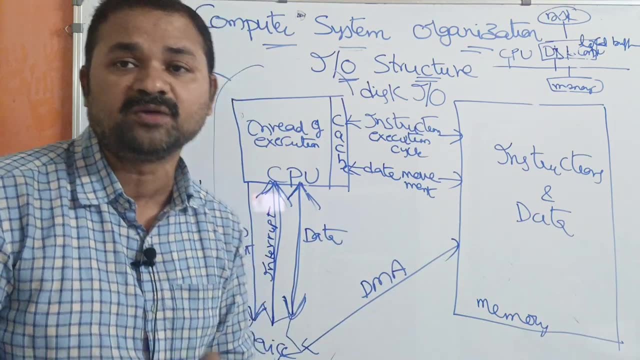 Whereas, coming to the IO request, IO will be towards the device Coming to the interrupt, IO will be towards the CPU. But here, what is the problem? here, What is the problem? The problem is this approach: interrupt initiated IO. 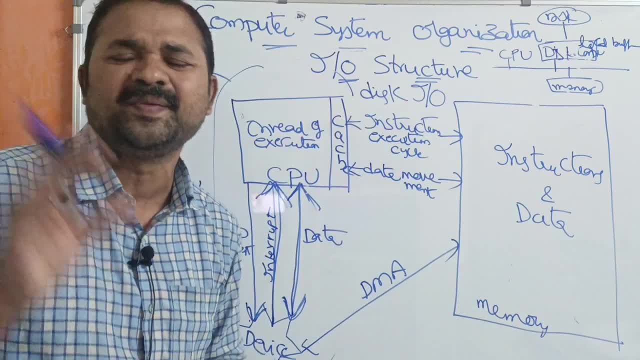 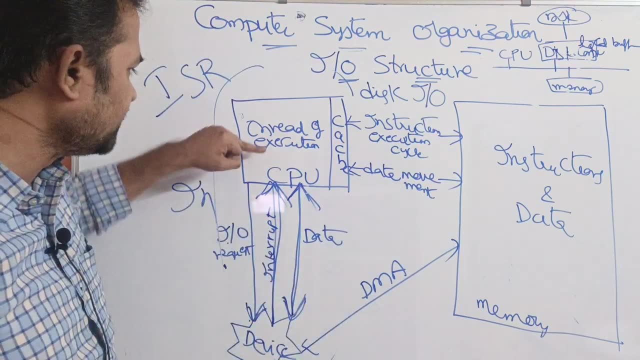 This approach is Suitable when we want to transfer small piece of information. If we want to transfer large amount of data, then this approach is not suitable. So let's see this one Here. CPU is executing the program. It finds an IO request. 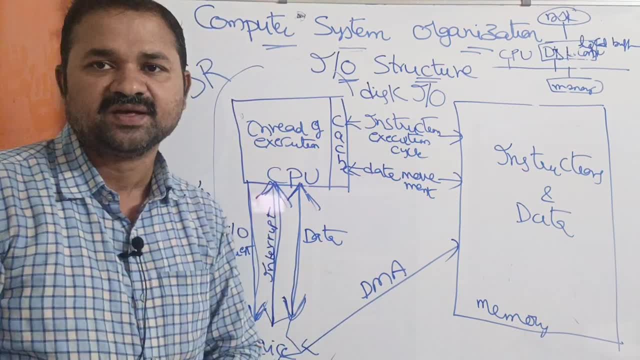 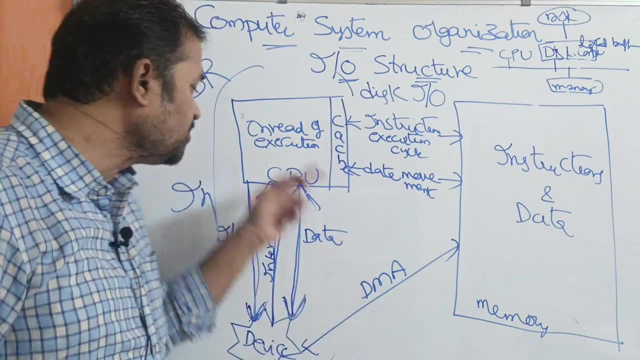 So CPU sends IO request to the device. So once the device has the data, then it will send an interrupt signal to the CPU. Now CPU will transfer the data from device to the main memory And, after execution, The 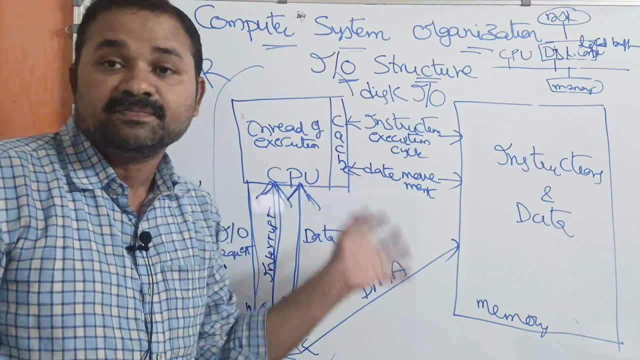 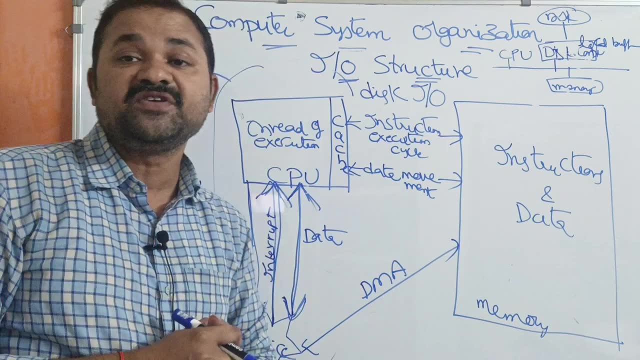 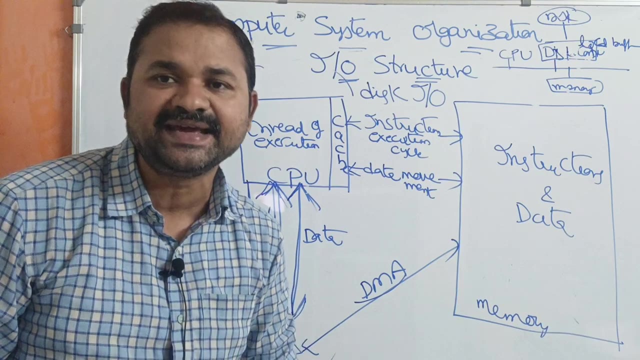 Data from main memory will be transferred to the device. This is about interrupt initiated IO. So this approach is suitable only for small piece of data transferring. If we want to transfer large piece of information, then we use DMA. We know that DMA stands for direct memory access. 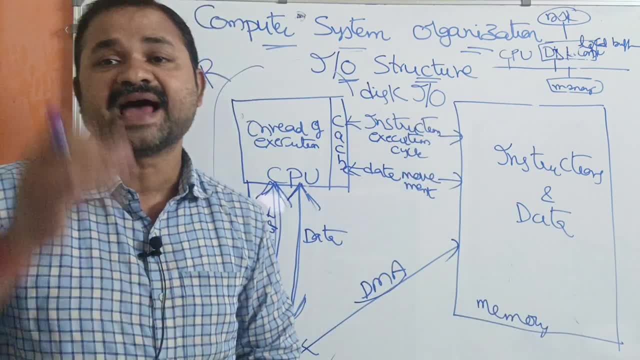 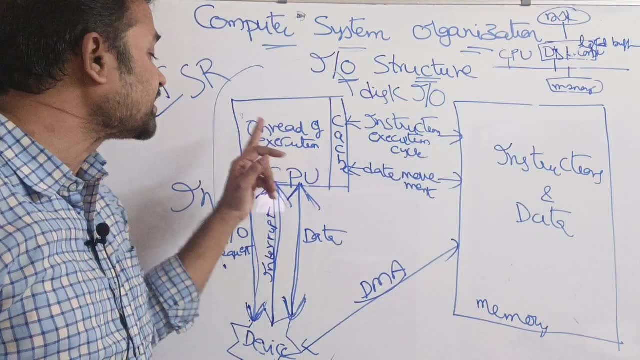 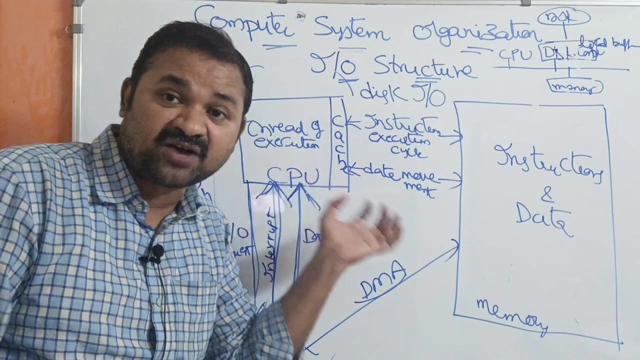 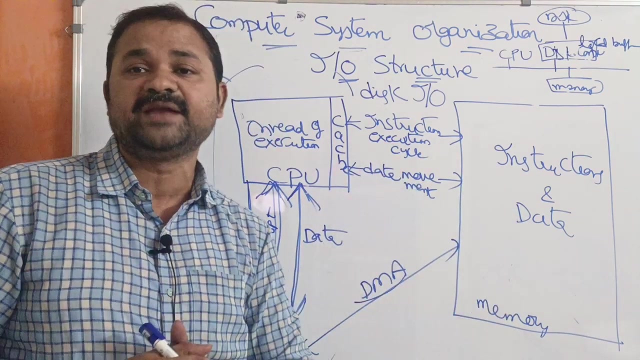 Here the responsibility of the DMA is it transfers the data from that device controller to the Main memory without CPU intervention. Here the task of CPU is in interrupt initiated IO. What is the task of CPU? It has to execute the program as well as it has to transfer the data from device to the main memory. 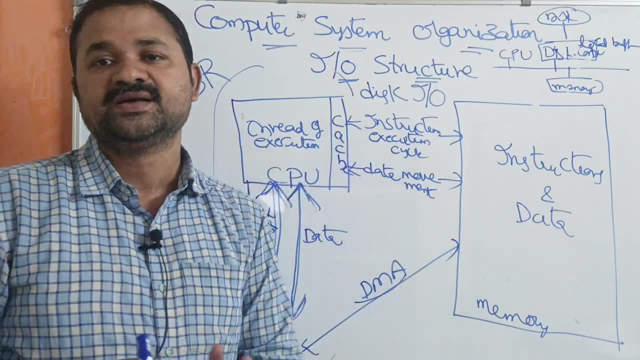 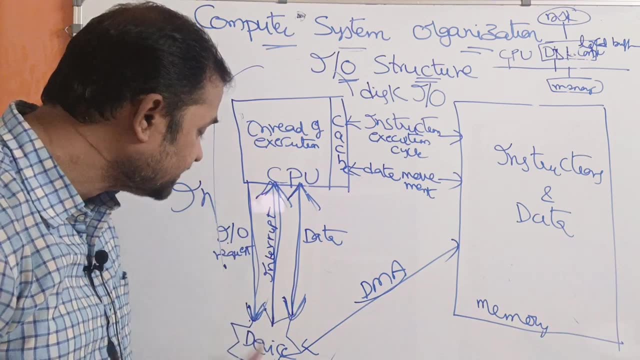 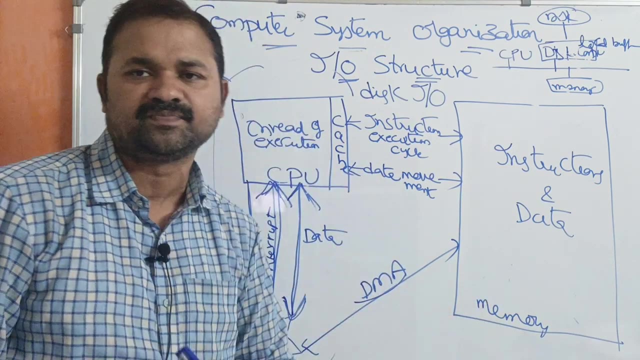 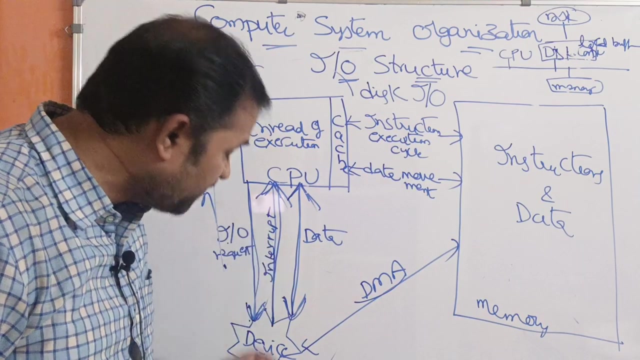 But now we are eliminating CPU intervention. CPU will focus only on executing the program, whereas DMA transfers the data from this device to the main memory without cpu intervention. so so cpu will focus only on its work, only the program execution, the dma solely responsible for transferring the data from device controller. 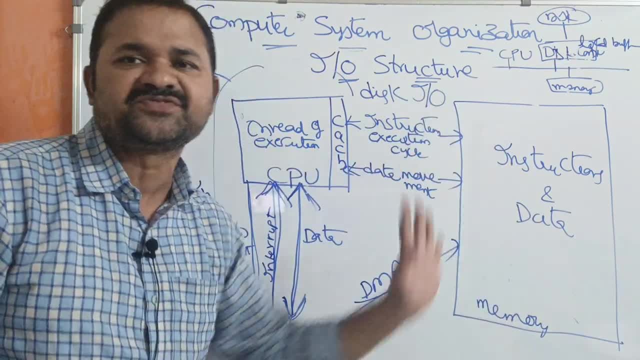 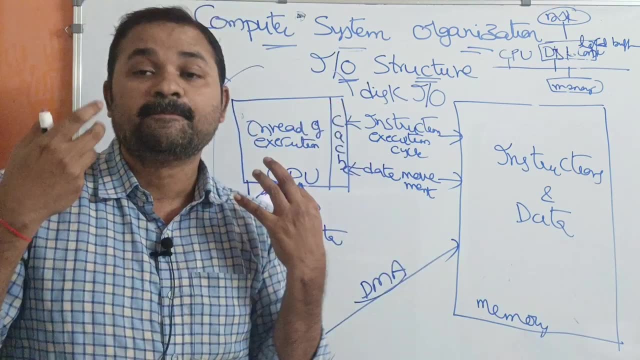 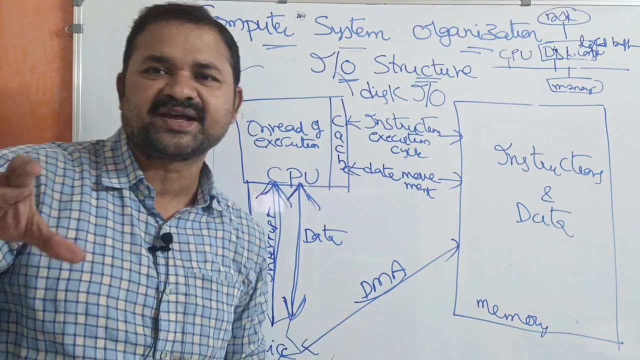 to the main memory. it has no other work, so it only transfers the data. dma is a high speed device, so by using dma we can transfer bulky amount of data from the device controller to the main memory. so this is about i o structure. i o structure means the name itself specifies the meaning: i o. 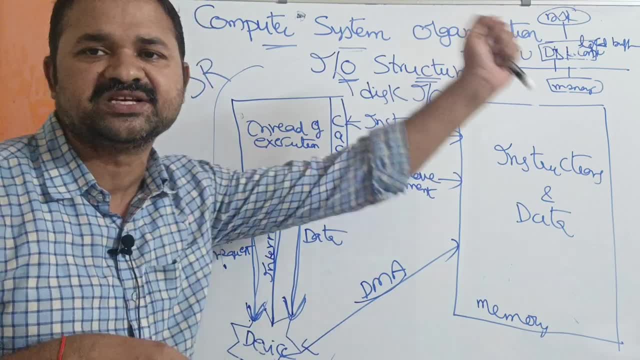 so how the data will be transferred from i o devices to the main memory.